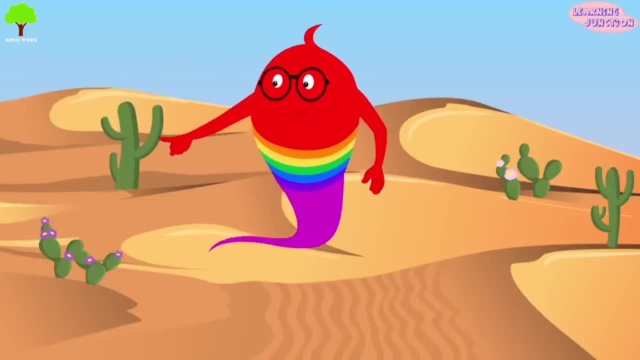 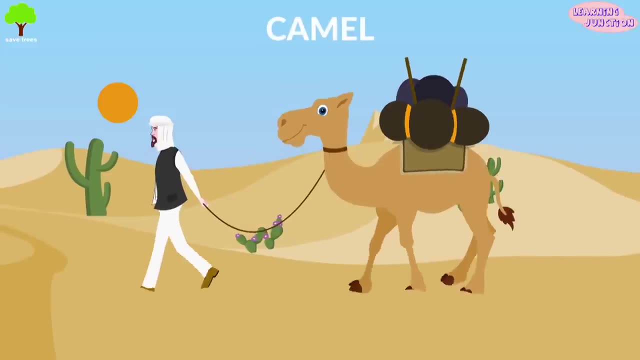 Let's learn about desert animals, birds and plants. Animals living in deserts have many special qualities and adaptations. Camel Camels are called ships of desert because they help in transportation. Their large feet helps to run fast, Their hair reflects the sun rays and 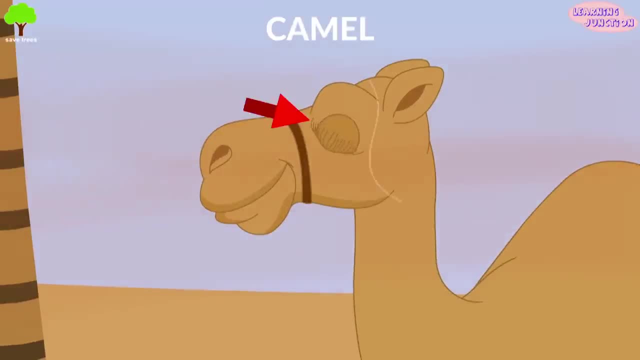 keeps them from getting wet. Their hair reflects the sun rays and keeps them from getting wet. Their fur is more dense than cool. Their fur is more dense than cool. Their fur is more dense than cool. Their bushy eyelashes protect from sand. Their bushy eyelashes: protect from sand. 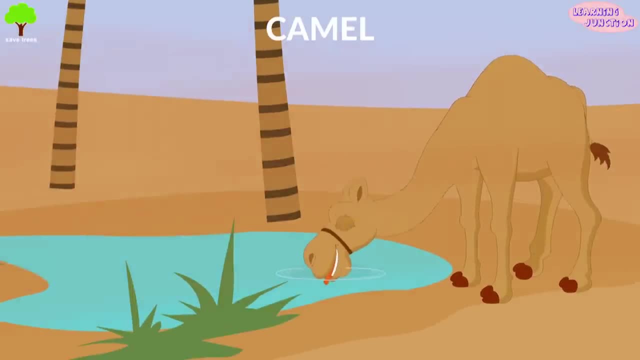 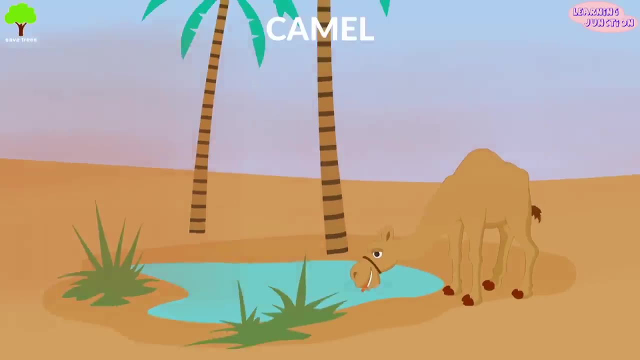 They can eat and drink in large amounts and store it as fat in the hump When no food is available. the fat converts energy in water. So this herbivore creature can live without water and food for many days. So this herbivore creature can live without water and food for many days. 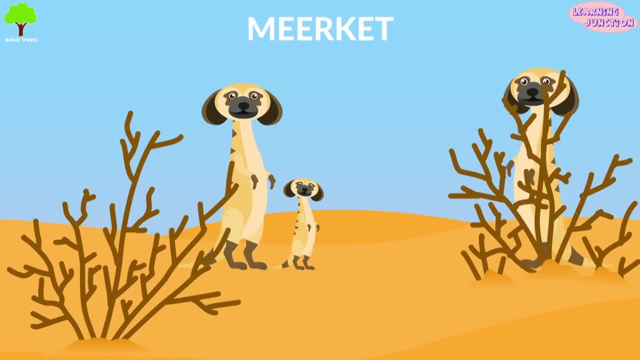 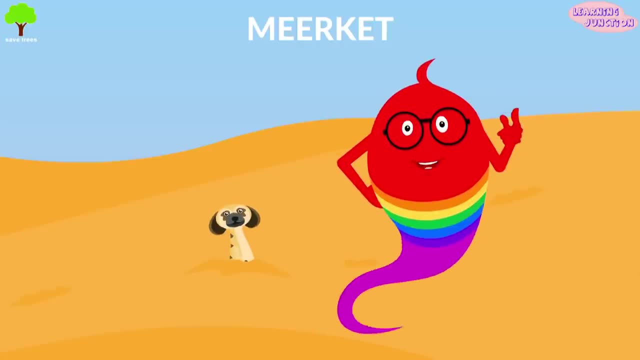 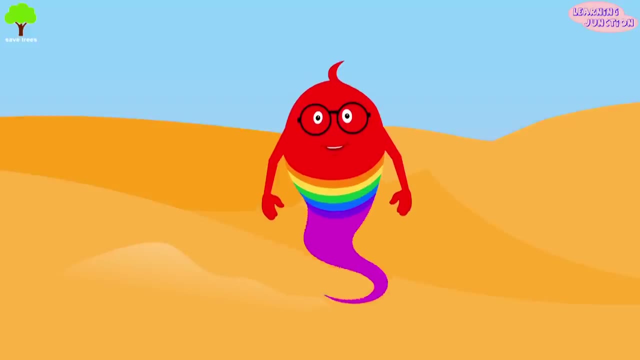 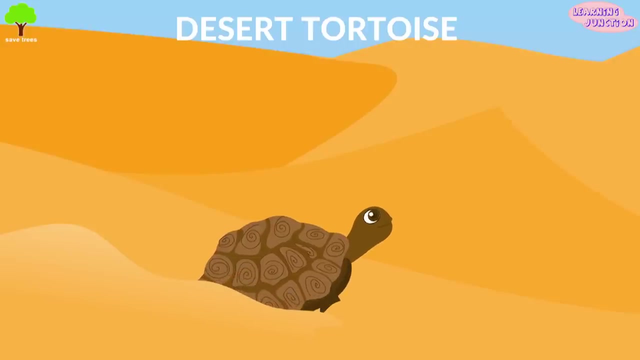 Meerkat. These cute omnivorous animals live in Kalahari Desert, Namib Desert and in South Africa, Africa. They dig large burrows to stay safe. Their brown and tan fur helps them to blend into the desert Desert tortoise. It lives underground in holes. This herbivore eats what's available in. 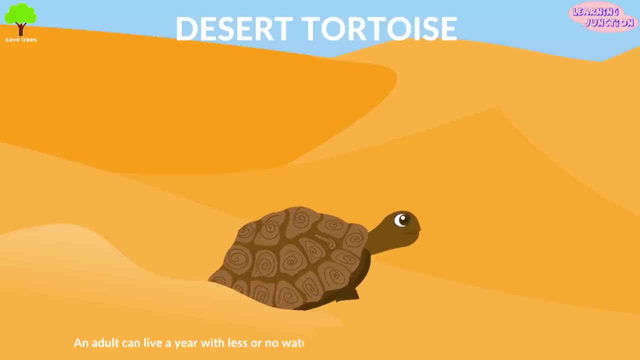 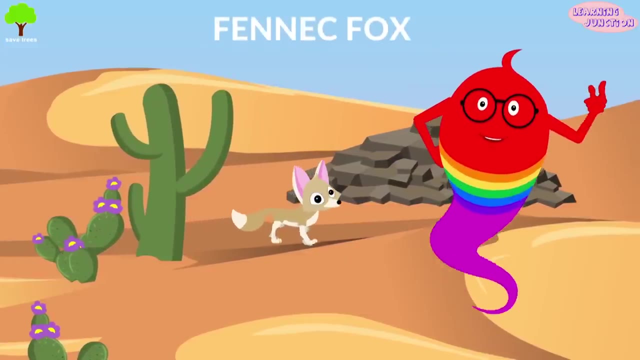 the desert. An adult can live a year with less or no water. It's found in the Sonoran and Mojave deserts. Fennec fox: It's the smallest of all the world's foxes. Their furs- keep them cool. 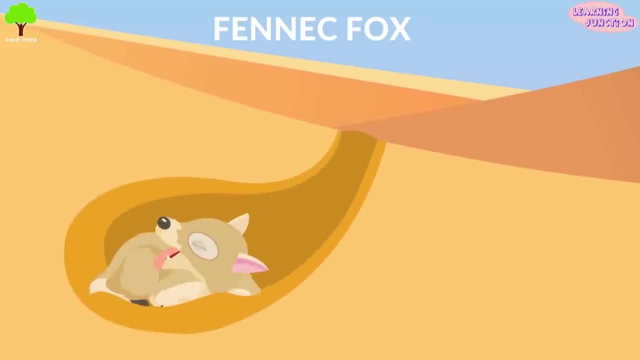 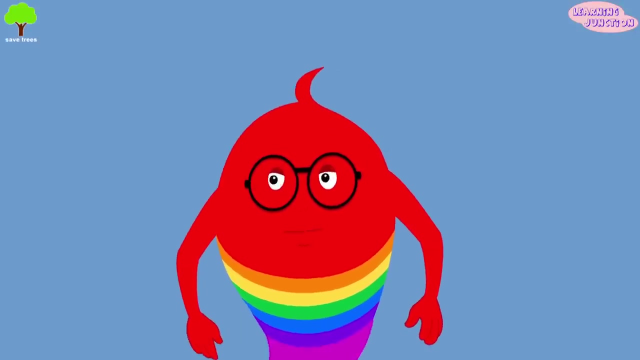 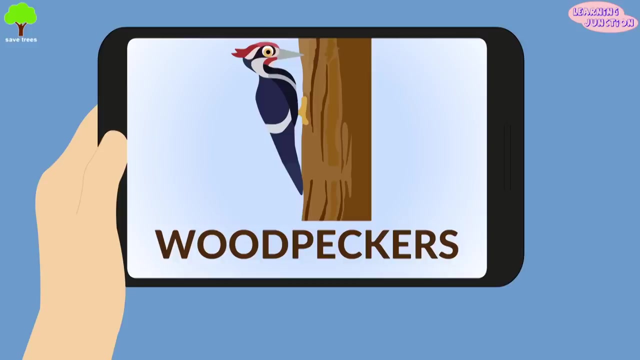 This nocturnal animal sleeps in underground dens to avoid hot sun. These omnivores need very little water. Examples of other desert animals: Coyote, rattlesnakes, deer, zebra, etc. Woodpeckers, roadrunners. 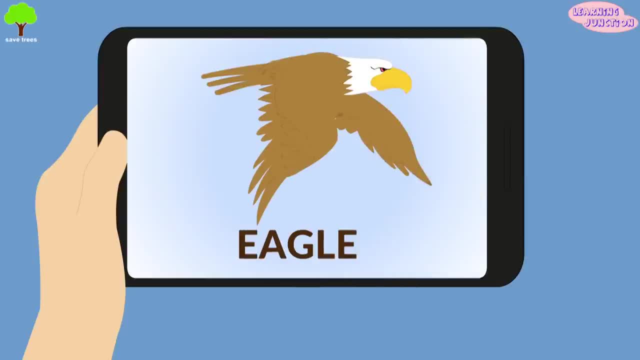 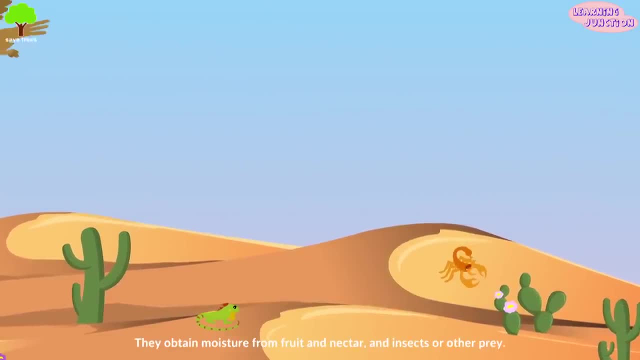 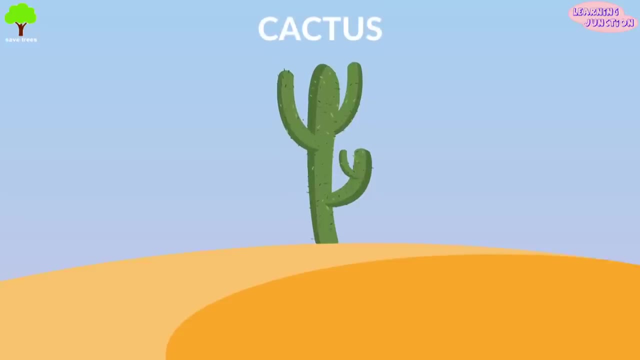 ostriches, owls, hawks and eagles are some desert birds. They obtain moisture from fruit and nectar, and insects or other prey. There are various types of plants which grow in deserts around the world: Cactus: The spines on a cactus help to protect it. Its roots are spread out to.